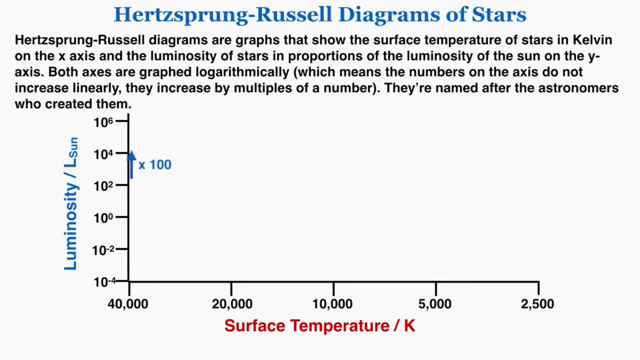 is multiplied by 100 from the previous notch, And on the x-axis, here, each additional notch is divided by two. The reason we graph HR diagrams this way is that this specific format allows us to see clear patterns emerging in the properties of stars. And just for context, this is the 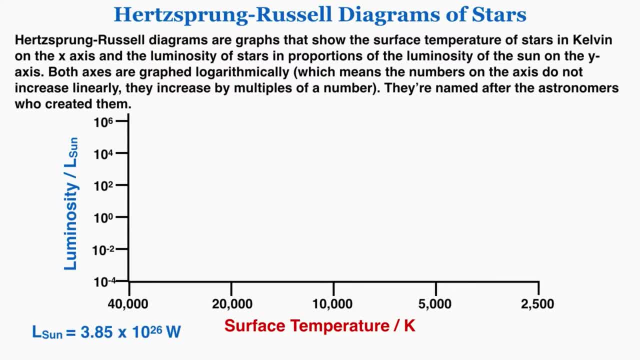 luminosity of the sun. So each notch on the y-axis is 10 to a certain power times that luminosity. If I were to take a large amount of stars from space at random and fill out this chart using the properties of those stars, it would look something like this: 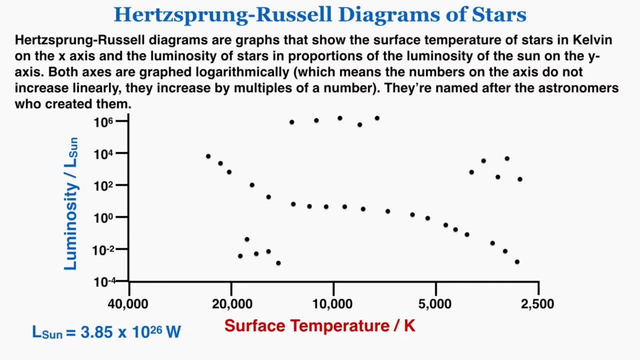 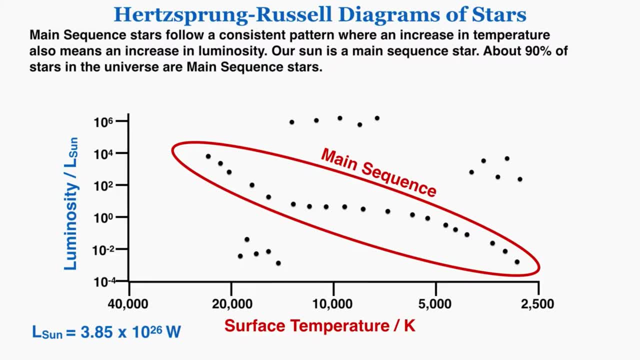 There are a few different patterns that emerge on this graph, so I'm going to go through and talk about them. The first pattern you might notice is this long streak of stars going roughly linearly all the way down the graph. These are called main sequence stars. 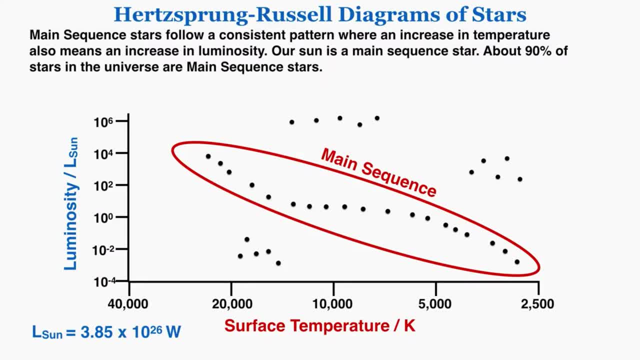 They're kind of the main type of star in the universe. They follow a line of stars that are in the middle of the graph and they're called main sequence stars. They follow a consistent pattern where an increase in temperature also means an increase in luminosity. 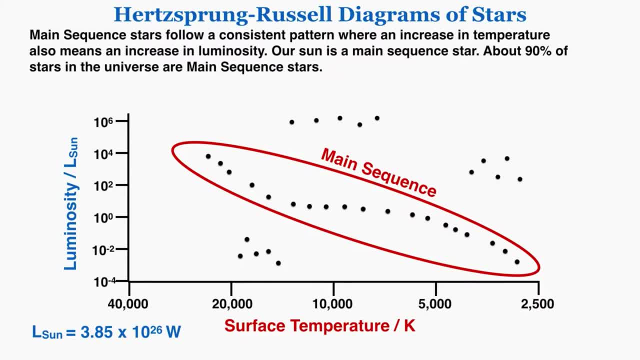 About 90% of stars in the universe are main sequence stars and our sun is actually also a main sequence star. So our sun obviously has a luminosity of one sun, of one earth sun. so that would be 10 to the power of zero for luminosity And that dot is roughly at the 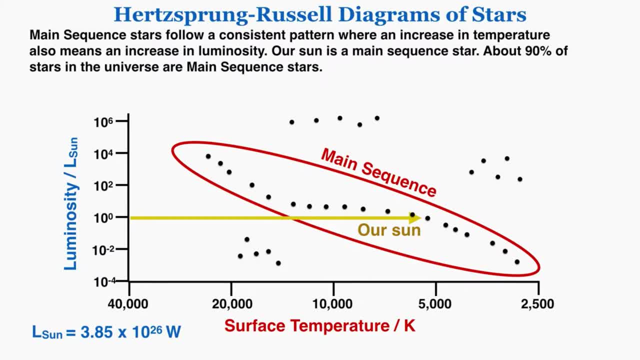 temperature of our sun as well. So that's where our sun would appear on this diagram. About 90% of all stars in the universe are main sequence stars. that's kind of why they're called the main sequence. It's the sequence of increasing. 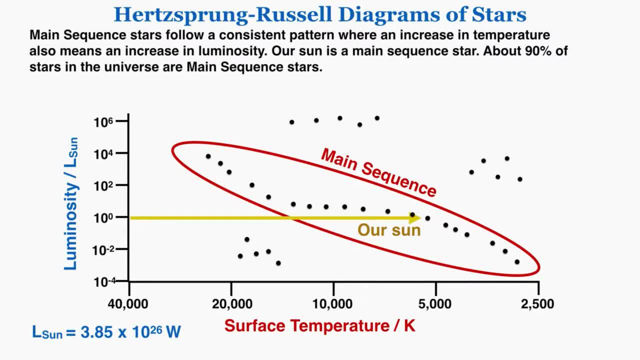 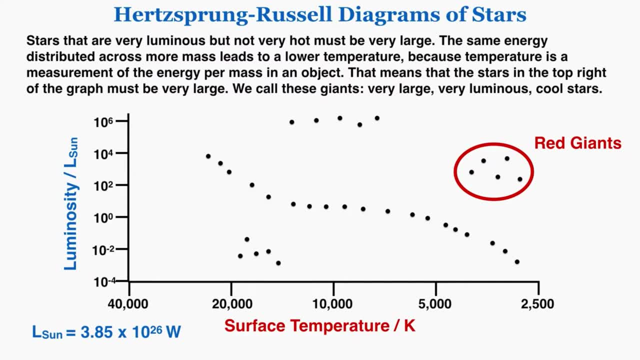 luminosity versus temperature that most stars follow. In this corner over here I can see that these stars are very luminous. They have a high luminosity number, but they're not very hot. This must mean that they're very large. The same energy distributed across more mass leads to a lower. 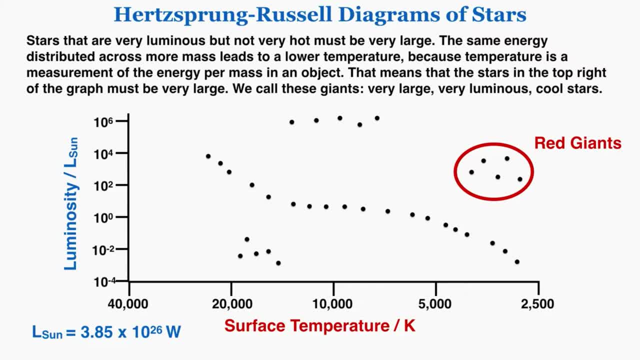 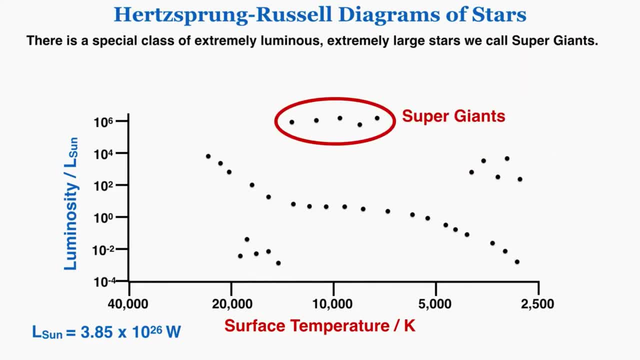 temperature. This means that the stars in the top right of the graph must be very large. We call these stars giants. They're very large, they're very luminous, but they're also relatively cool. There's a special class of extremely luminous and extremely large stars that we call super. 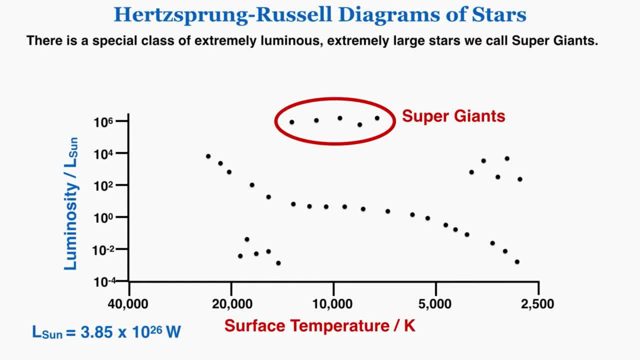 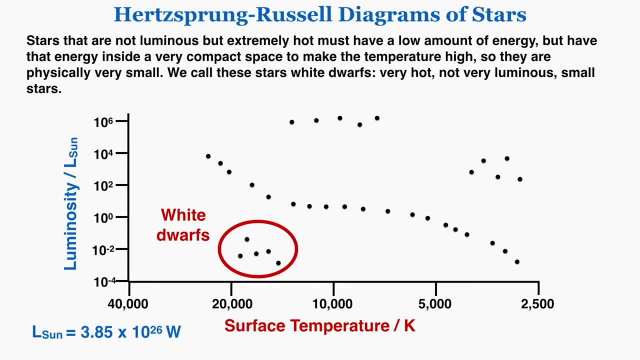 giants. So this would be the area of the HR diagram where they appear. Stars that are not too luminous but are extremely hot must have a low amount of energy but have that energy inside a very compact space to make the temperature high. So they're physically very small. We call these stars white. 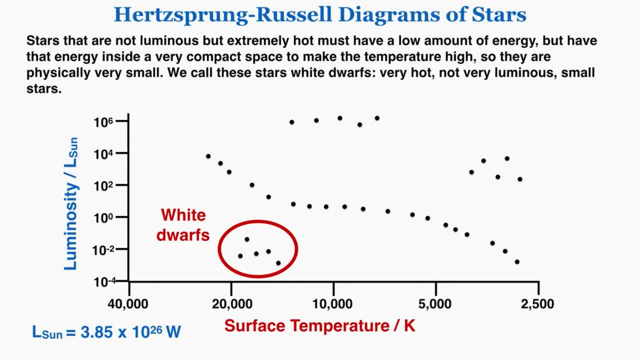 dwarfs. They're very hot, they're not very luminous and they're small stars. So in general we say that stars on an HR diagram exist. along the surface of the diagram, They appear to be just as small as the stars in the data. 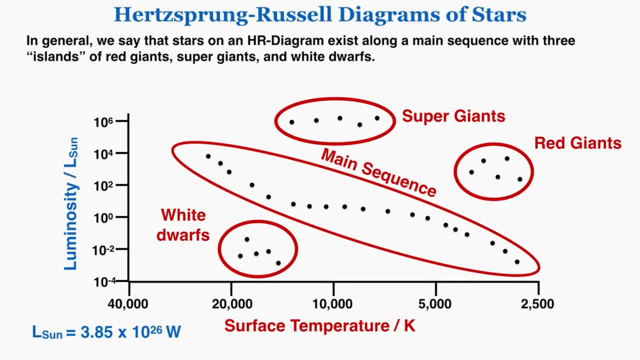 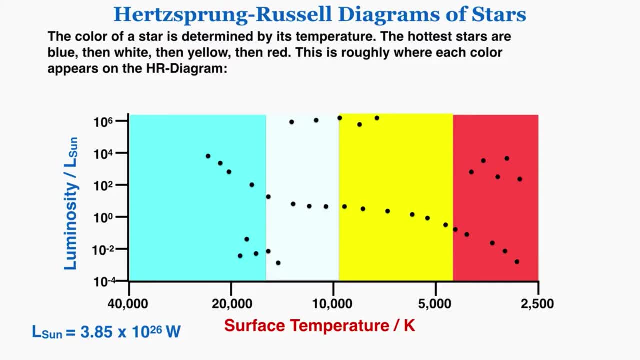 a main sequence with three islands of red giants, supergiants and white dwarfs. The color of a star is determined by its temperature. The hottest stars are blue, then white, then yellow, then red, and this is roughly where each color appears on the HR diagram. So any stars that have a temperature of 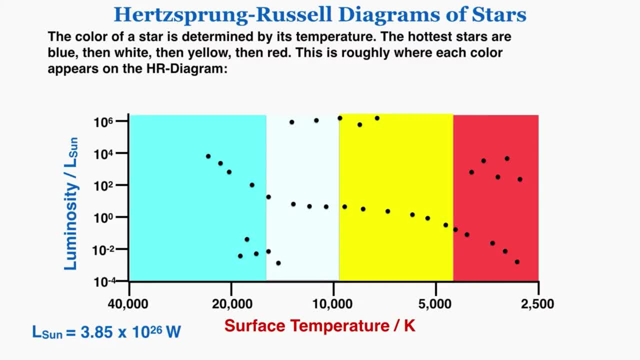 roughly 10,000 to 5,000, Kelvin will appear as yellow. From about 13,000 to 10,000, they'll appear as white, and from 40,000 to 20,000, it's blue, and from less than 5,000, those stars appear. 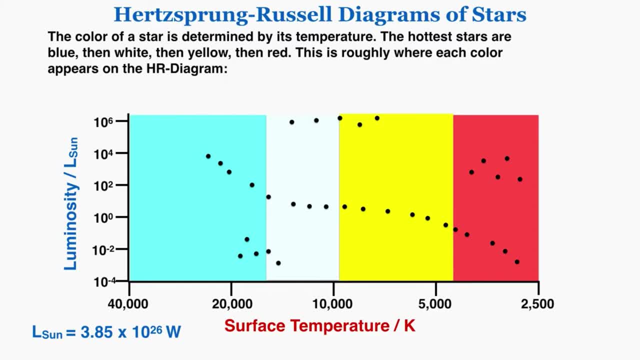 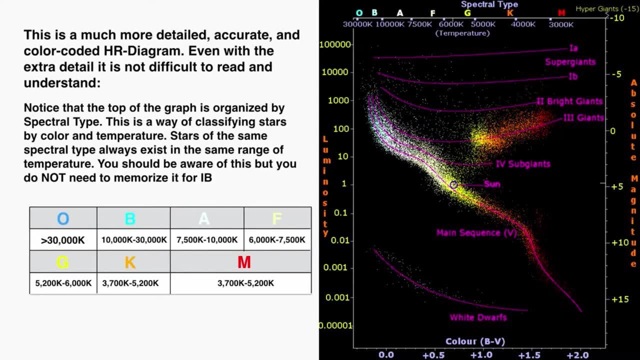 as red. So if a dot falls within that color band, that star literally is that color in the sky. This picture on the right is a much more detailed, accurate and color-coded HR diagram and even with the extra detail it's not too difficult to read and understand. So I can see. 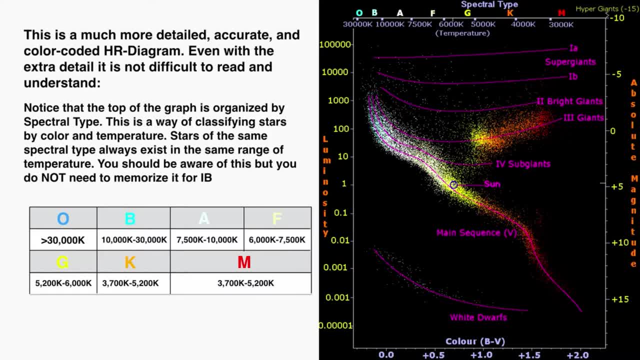 that I have that main sequence of stars going up and to the left I have a patch of white dwarfs on the bottom left, I have giants on the top right and supergiants on the top and you can see that the axis on the left measures luminosity in terms of multiples of the. 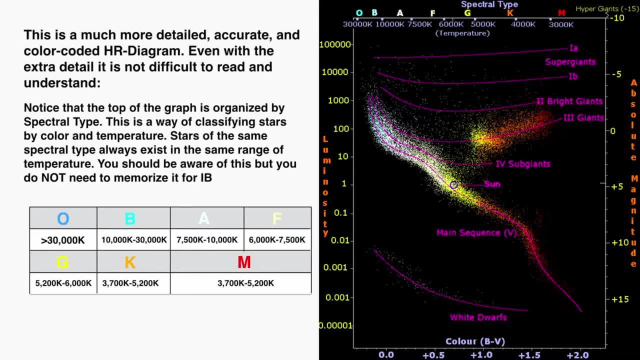 sun's luminosity and on the x-axis listed on top you can see temperatures listed. The top of the graph is also organized by spectral type. This is a way of classifying stars by color and temperature. Stars of the same spectral type always exist in the same. 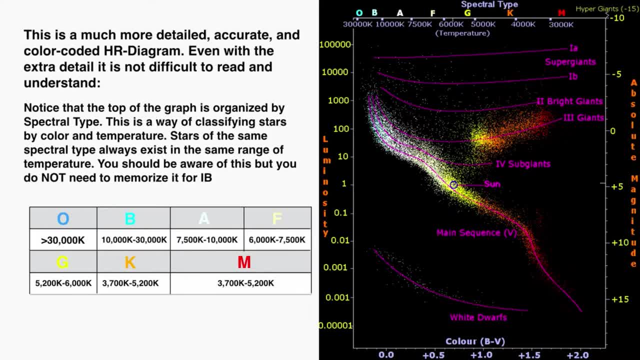 range of temperature. You should be aware of this, but you do not need to memorize it for IB physics specifically. So I've listed the different spectral types. The names of the spectral types are really just names for ranges of temperature and the color that the stars appear as. 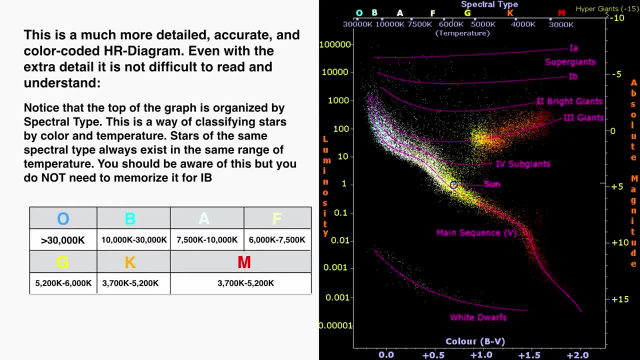 The letters are O, B, A, F, G, K, M, and you can see, each one corresponds to a different color of star and a different range of temperature. So if a star is spectral type B, its temperature must be between 10,000 and 30,000 Kelvin. If it's spectral type K, it must be between 3,700 and 5,200. 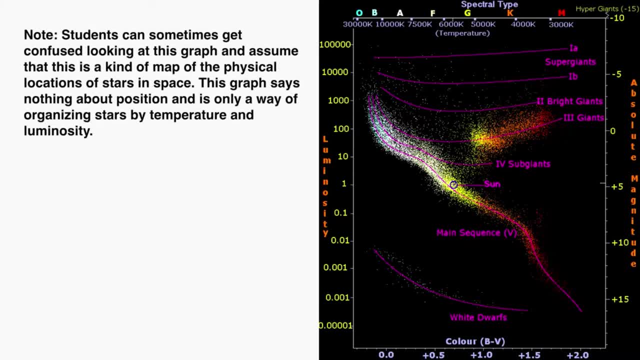 Kelvin. And just as a note, students can sometimes get confused looking at this graph and assume that this is a kind of map of the physical location of stars in space. Like it looks like it could be like a strangely shaped cloud of stars, But this graph says nothing about the position of stars and 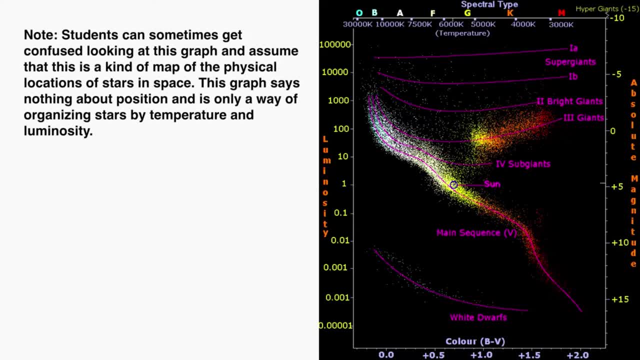 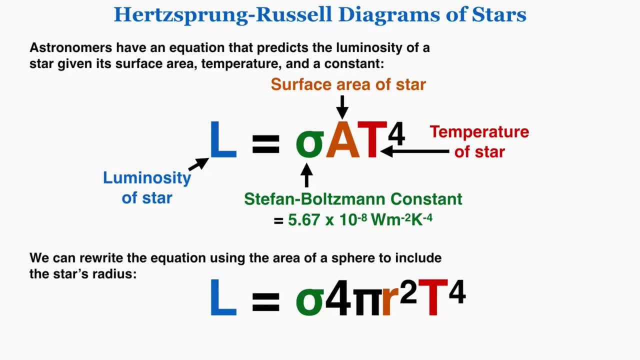 is only a way of organizing them by temperature and luminosity, So this says nothing about where stars physically are in space. Astronomers have an equation that predicts the luminosity of a star given its surface area, temperature and a constant. I'm just going to have you read through. 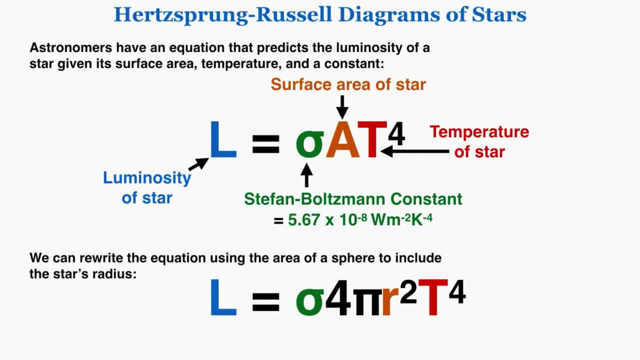 this equation. It's pretty straightforward. There's one new constant that we haven't worked with before, the Stefan-Boltzmann constant, which is 5.67 times 10 to the negative 8 watts per meter into the negative. fourth, Because all stars are spheres, we can rewrite that surface area as the. 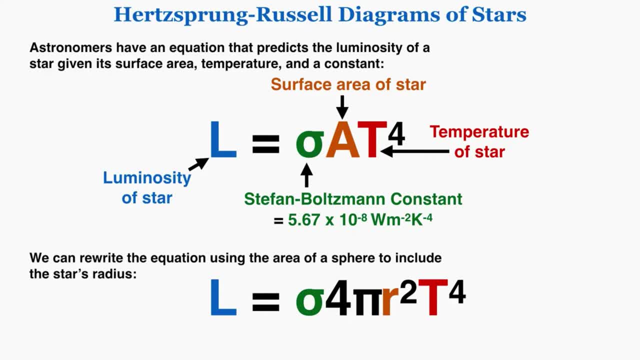 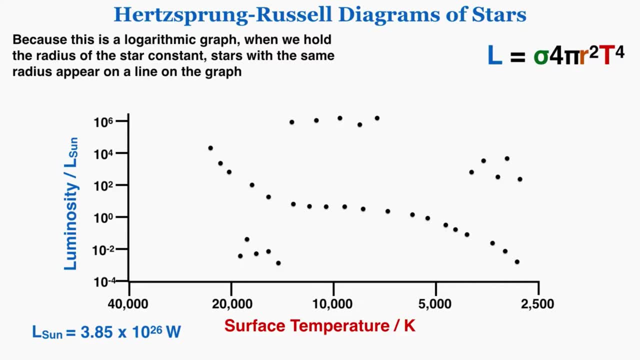 surface area of a sphere. to get the bottom equation that includes the radius of the star, And because this is a logarithmic graph, when we hold the radius of the star, constant stars with the same radius appear on a line on the graph. So, as an example, any star that appears exactly on 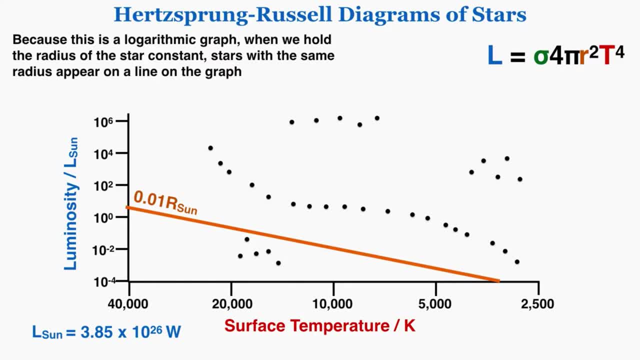 this line has a radius of about 1 100th of the radius of Earth's sun. Stars that appear on this line have a radius that's equal to Earth's sun, and stars that appear on this line have a radius that's 100 times larger than Earth's sun, And you could draw these lines for any radius that you. 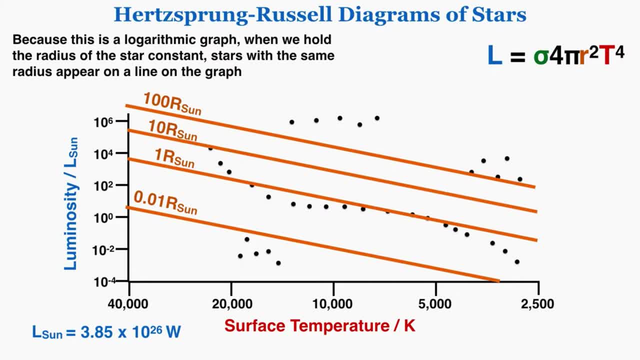 want As an example, between 1 and 100, you could find a line for 10 times the Earth's sun. but we don't want to fill this up completely with lines because we could draw an infinite amount, So I'll just draw a few as an example. So we call these lines of constant radius Any two stars that. 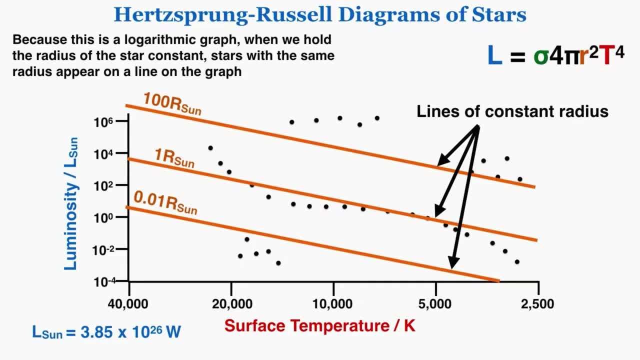 appear along the same line of constant radius, have the same radius as each other. So you can see that as you go up and to the right on the graph, the radius of the stars that you're looking at- therefore, the size of the stars that you're looking at- increases This equation: luminosity. 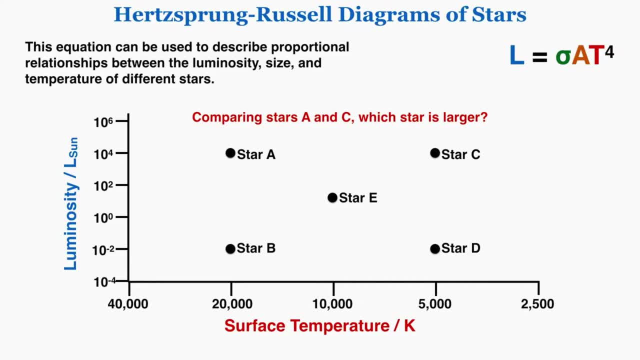 is equal to the Boltzmann constant times, the area times, the temperature to the fourth, can be used to describe proportional relationships between the luminosity size and temperature of different stars. I'll use this to answer a few questions about the sizes of different stars on this HR. 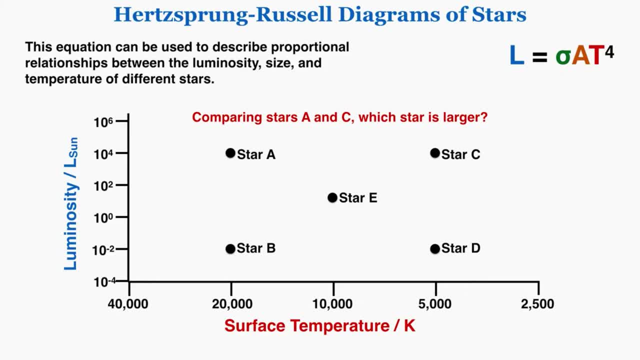 diagram. This first question says comparing stars A and C. which star is larger? So I can see A is in the top left, C is in the top right. I can compare their luminosity and see that they have the same luminosity. they're on the same point on the graph And I can compare. 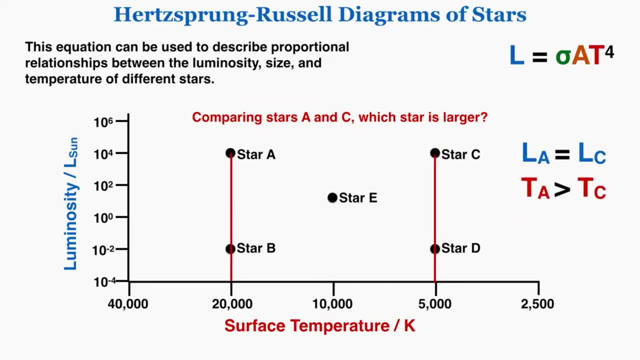 their temperatures and see that star A has a greater temperature than star C. If I take that equation for luminosity on the top and rearrange it to find the surface area of a star, this is the equation that I get. So because star A and star C have the same luminosity but star A has 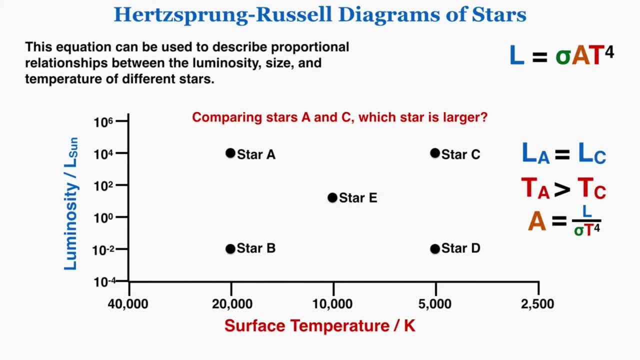 the same temperature, the denominator of star A's area will be greater than the denominator of star C's area. The numerators are the same, but there's a number in the denominator of A that is bigger than the denominator of c. So if you have a bigger denominator, that means that as a whole. 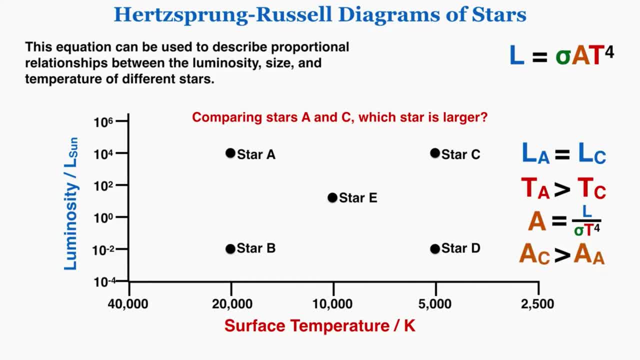 your number is smaller. So that means that the surface area of C is greater than the surface area of star A, Which means that star C is larger than star A. So to get that information I used information from the diagram and the equation L equals the Boltzmann constant times, area times, the 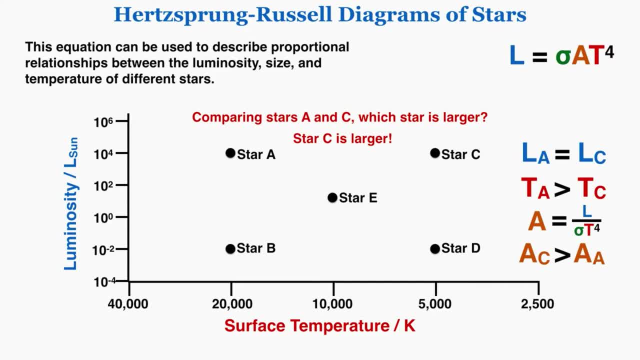 constant times, area times, temperature to the fourth. So, based on that pattern, following a horizontal line from left to right on an HR diagram leads to larger stars. This fits our understanding because if we look back here we can see that as we go from left to right, we do get. 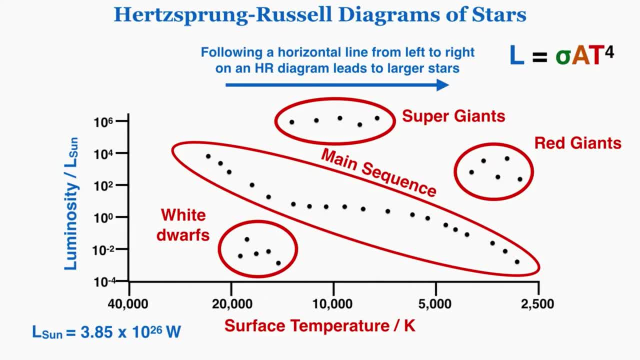 larger and larger stars. The red giants are to the right of supergiants, but they're also lower on the graph. If you were to just follow a perfectly horizontal line from the supergiants, you would get larger and larger stars in that direction. So if you draw any horizontal line between two, 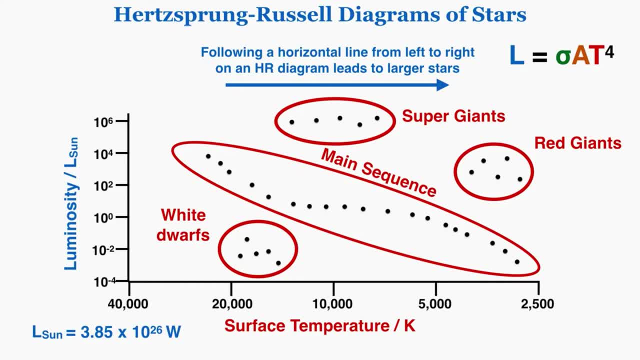 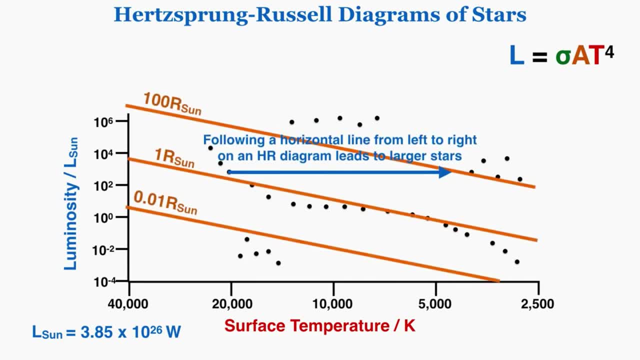 stars on this graph and two stars are on the same horizontal level. the star on the right will always be bigger than the star on the left. This also fits our understanding based on those lines of constant radius. I can see that as I go from left to right, the radius is increasing. We can 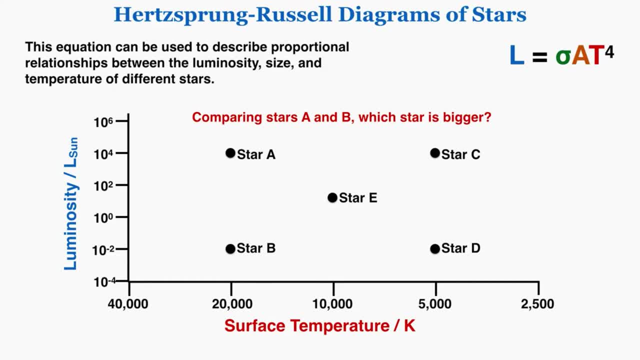 now try comparing stars A and B and see which star is bigger here. So star A and B. star A has the greater luminosity And both stars have the same surface temperature. Plugging that into the equation for area: if the denominators are the same but the numerator of A is bigger than the numerator of B, that means that